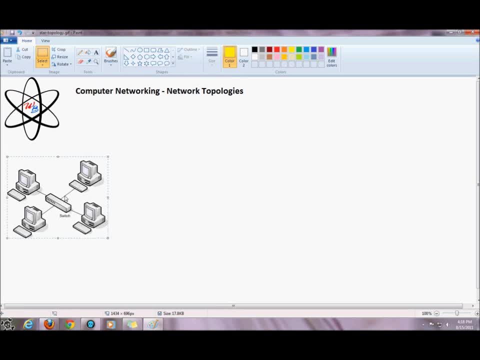 now our star topology. how this works is that all devices on all devices or nodes on the network are connected to a central device called a hub or, in this case, a switch. now, if a machine, whenever a machine, is sending information, that information is sent to the central device, the switch and the 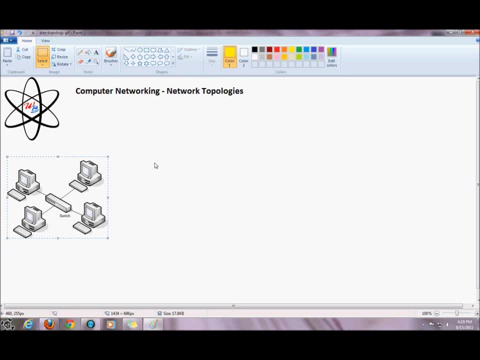 switch broadcasts that information to the central device, the information to out all other ports except the port that it received the information on. what that means is that if this machine is this machine, this machine is sending information to this machine, then it's an information to the hub. the hub broadcasts in the information out all the ports except. 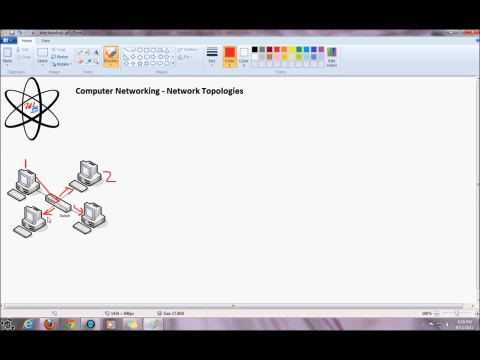 the port that you receive the information from, see that information was not intended for this machine or this machine. these machines are discarding information and machine to it will accept and do whatever it wants with the information. or second topology is bus topology. now, with the bus topology, all devices, oops. 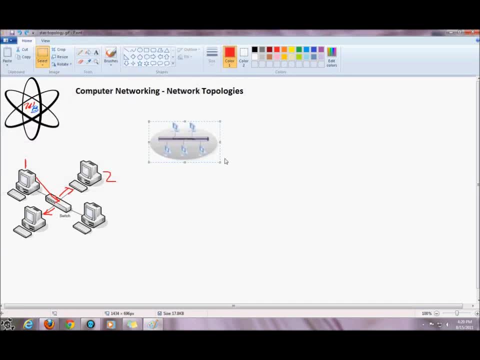 the bus topology. all devices, all the nodes are an interlock, are connected to a backbone. this is therite, is the backbone. the backbone has something on it called terminators. the terminators really cut transmission. it prevents transmission from going any further this way or this way. because how the bus works is that when a 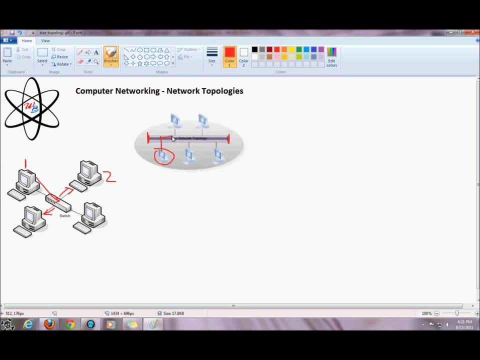 machine uh transmit information under the backbone. information is sent right along the backbone. each machine, each node checks that information to see if it's actually addressed to them. if it's not addressed to them, they just leave it alone. um, whichever information, whichever node destination node that, whichever node destination know that the information is intended for. 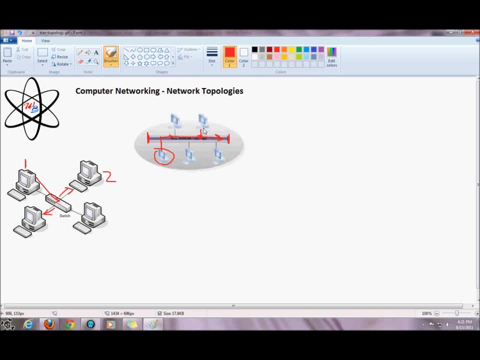 that node will take off the information of the backbone, information from the backbone. now if, for some reason, the node, the desk they know that the information is intended for, is not on the network for some strange reason, then the information will travel right along the backbone until it hits a terminator. 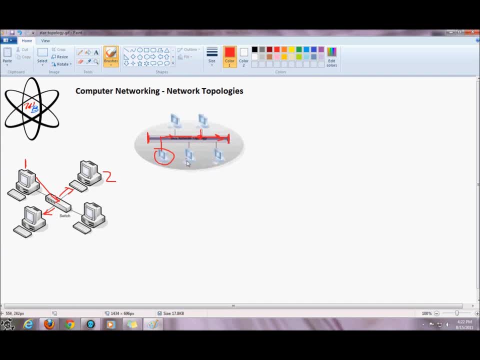 and information is just discarded, and that's the purpose of the terminators. uh, our other topology is the network. now with the ring, each device is each device on the network. each node on the network requires a special permission card, called a token, before they can send information. if a node does not have the token, it cannot. 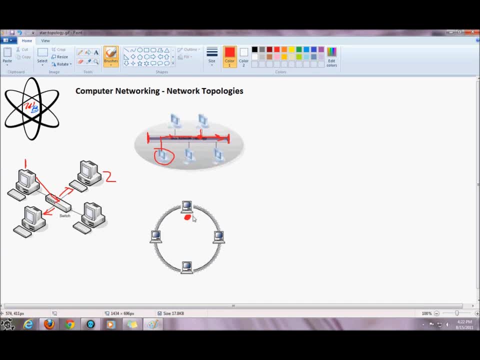 send information on the ring network. so, seeing that this machine has their token, then you can transmit whatever information it has to whichever machine on the network after the machine, that is, it has transmitted information to receive the network, it would the machine. the sending machine will just discard the token. 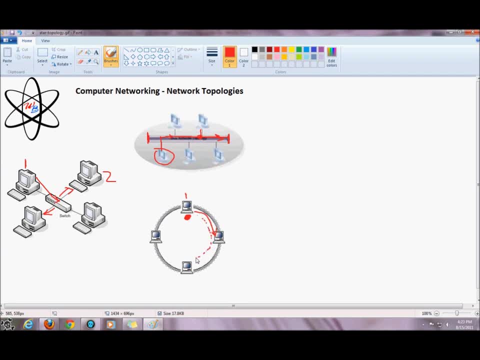 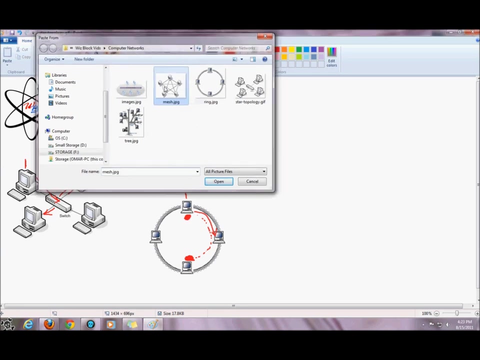 and the token would float around the network until another node on the network picks up the token pixel to be able to transmit its information. so the in the ring topology nodes can only transmit information on a network when they have the permission card or the token. other network are we looking at is the mesh topology, now the 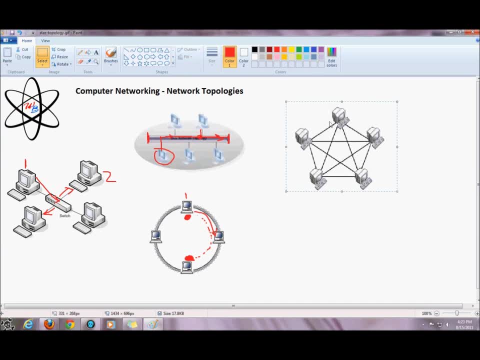 mesh topology is really nodes that are connected via redundant links. I think that's pretty self-explanatory. but each node has several roots or links connecting it to other nodes on the network. so in case one node goes down, then the there are several other backup links and, last but not least, we have a. 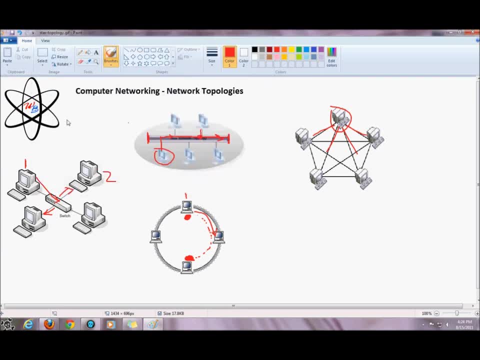 hybrid topology known as the tree. now, the tree is comprised of bus topology or bus topology devices connected to the bus and the tree- I'm sorry, a star. so this is a central device, or the hub, and each device is connected to it, to the central device. that's how you know that it's a star. 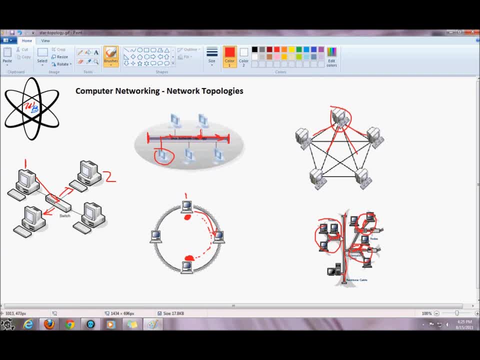 once the nodes are connected to a central device, it's a star, and that star is connected to the backbone and you know that devices that are connected to our backbone, they are. you know that the ball is known as a boss. yes, and that's it, you guys. 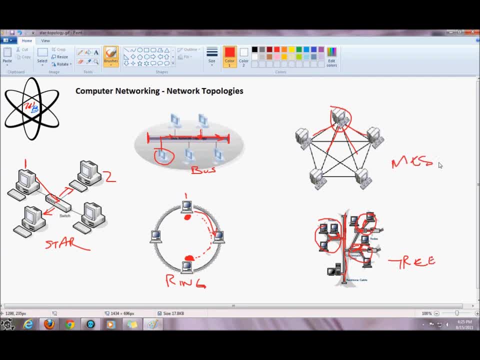 tree mesh. the real disadvantage that with the star is that if this, if the central device goes down- let's say the home, you know that the central device goes down, let's say the home, you know that the central device goes down, let's say the home goes down, then the network will feel because the hub is really what keeps a. 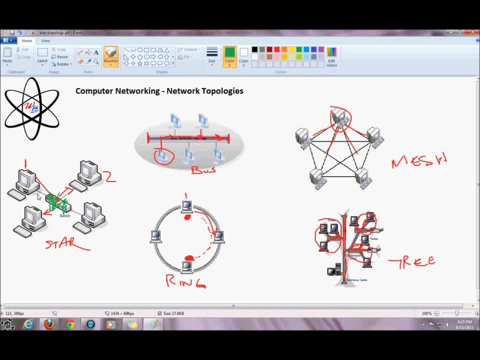 network in place. it allows information to transmit from sender to receiver. that's the same thing with the bus topology. if the backbone breaks then the entire network goes down. same thing with the ring. if one node on the ring goes down then it can hamper this transmission of information. let's say this machine.